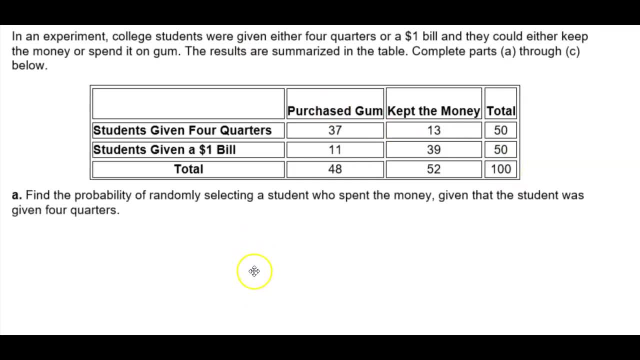 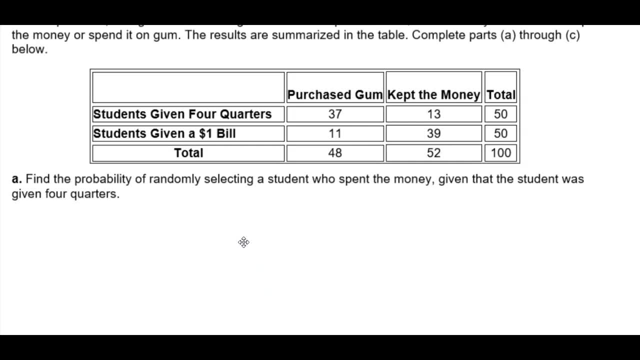 to give us a total of 100. Now what we want to do is find the probability of randomly selecting a student who spent the money, given that the student was given four quarters, Now spent, the money is going to be purchased the gum and the student that was given the four quarters is the following row there, and how. 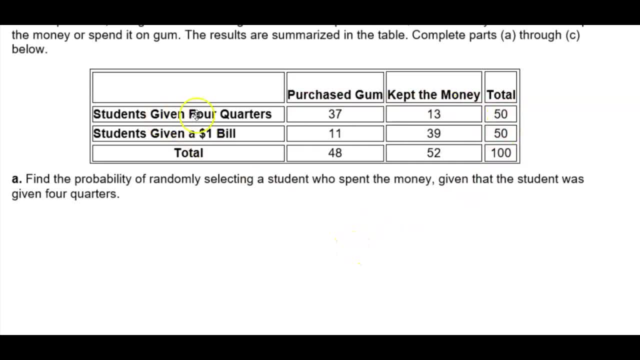 many are there as a total. So look at the student that were given the four quarters. There were 50 total, and then the student that was given four quarters that purchased gum were 37. Now the conditional probability of B occurring, given that A has occurred, can be found intuitively. 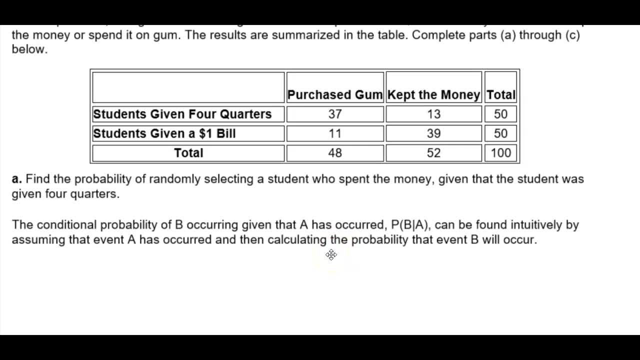 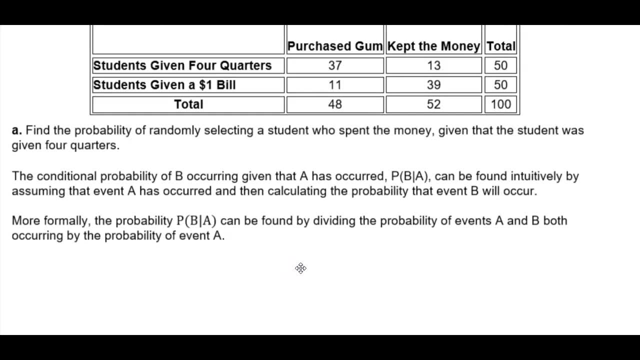 by assuming that event A has occurred and then calculating the probability that event B will occur. Now, more formally, the probability can be found by dividing the probability of events A and B, both occurring by the probability of event A. So we would have the probability of event B provided. 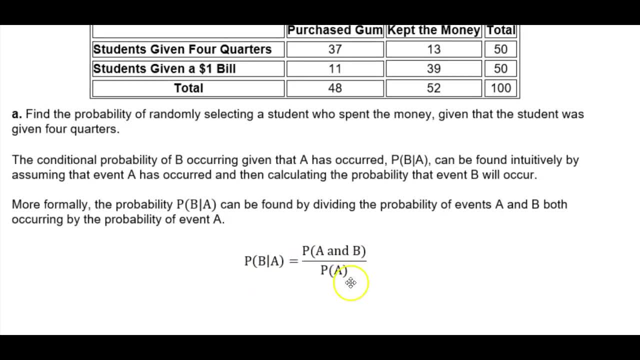 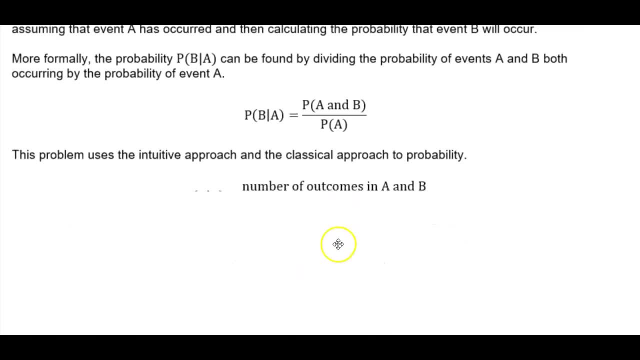 A has occurred is equal to the probability of A and B divided by the probability of event A. Now, this problem uses the intuitive approach and the classical approach: probability. So the probability of event B, provided that A has already occurred, is the number of outcomes in A and B divided by the number of outcomes in A. Now, in this case, given four quarters, 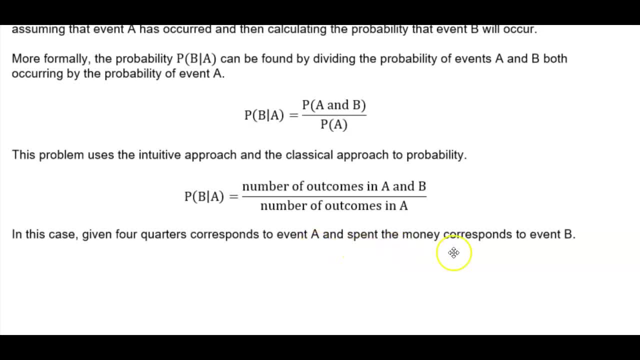 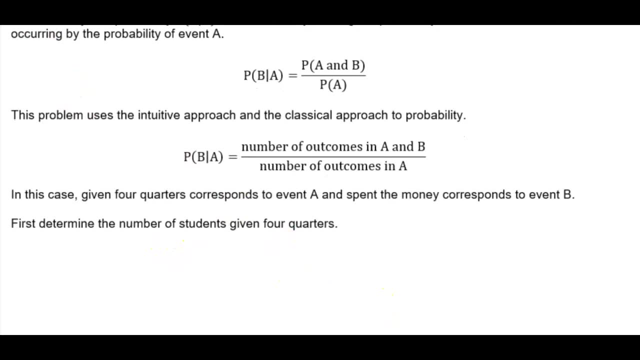 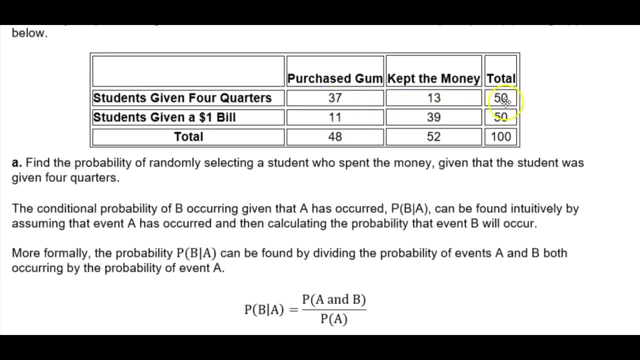 corresponds to event A and spent the money corresponds to event B. So we need to first determine the number of students given four quarters. Well, that's 37, 13, which is equal to 15 students. so 37 plus 13 gives us 50 that were given four quarters. 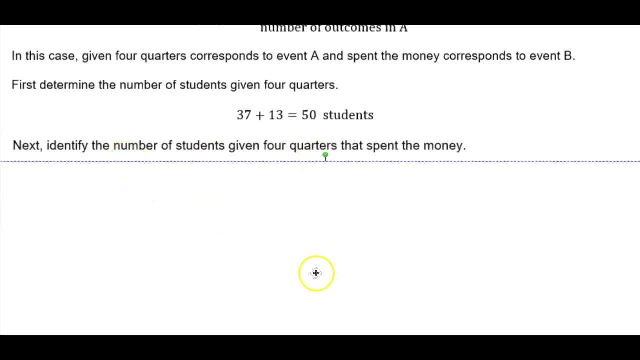 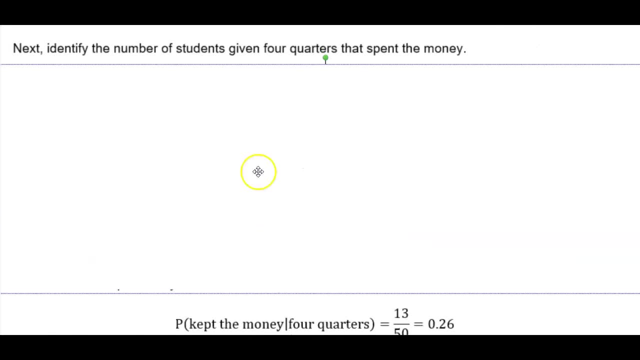 now identify the number of students given four quarters that spent the money. well, the students that get were given four quarters that purchased gum were 37, so therefore 37 students. now we're going to calculate the probability. so the probability that the students spent the money, given that they were had four quarters, is 37 over 50, which is equal to 0.74. 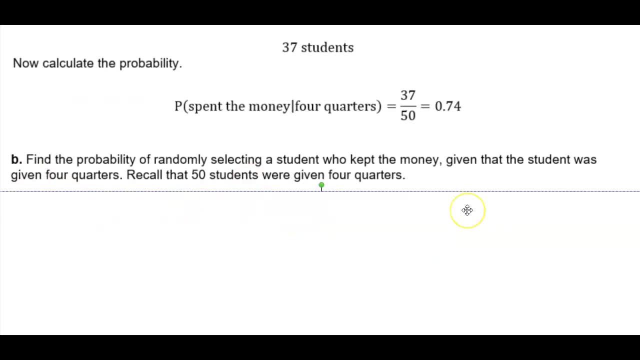 now we want to find the probability of randomly selecting a student who kept the money, given that the student was given four quarters, and recall that 50 students were given four quarters. so now we need to look at the value that the students who kept the money. well, if we come,